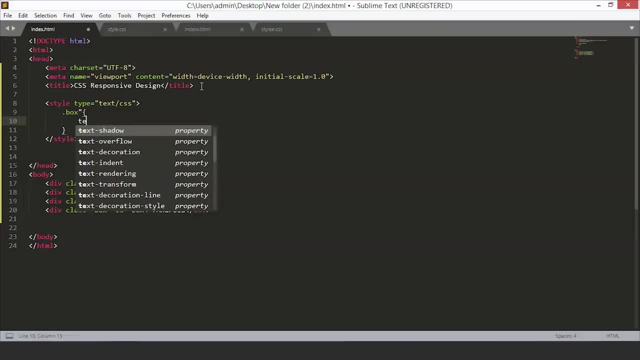 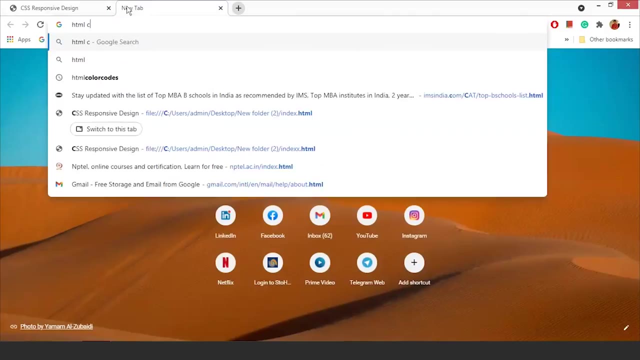 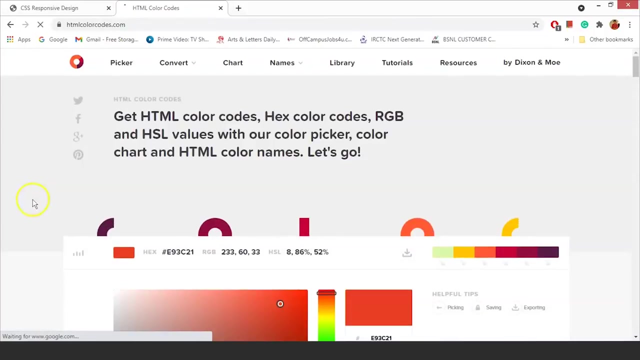 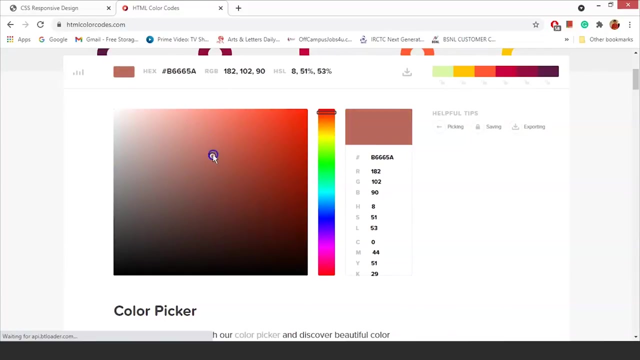 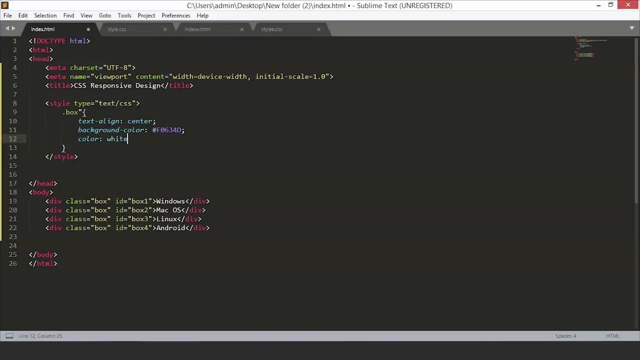 And we'll text align. we'll send the text aligned to center. We'll touch on recon-need-picklehuman. We will set the background color. let's select some color. so we go to this html color pools. choose a good color. let's select this color. it looks good. we set the text color to white. 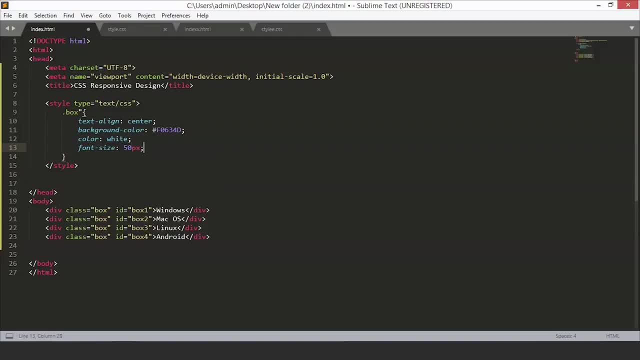 and we will set the font type to say something typical and just save the file. let's go back and refresh the page. We have some color, let's figure it out, ok. so first, so it's not valid, let's do this. 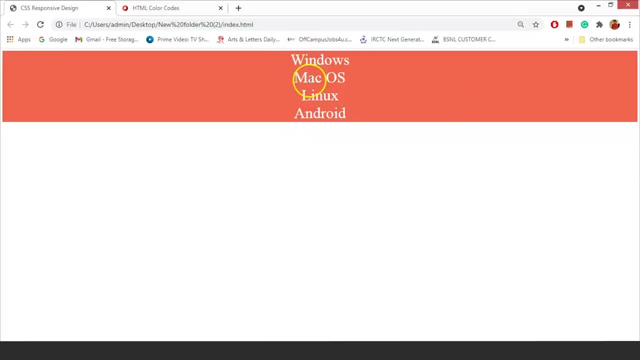 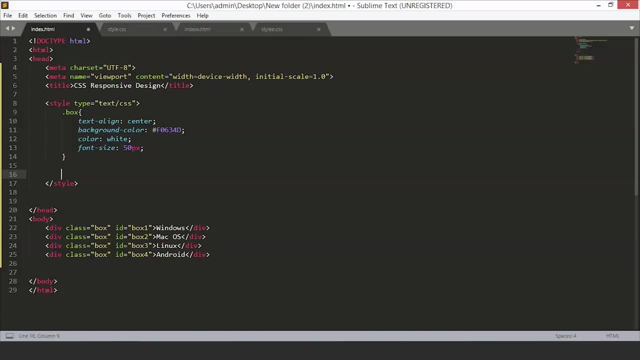 so now, if you refresh, you see we have our divs with Windows, Mac OS, Linux and Android and with this background color. So to design a responsive web pages, we use the media queries. so what are media queries? let's first discuss this. 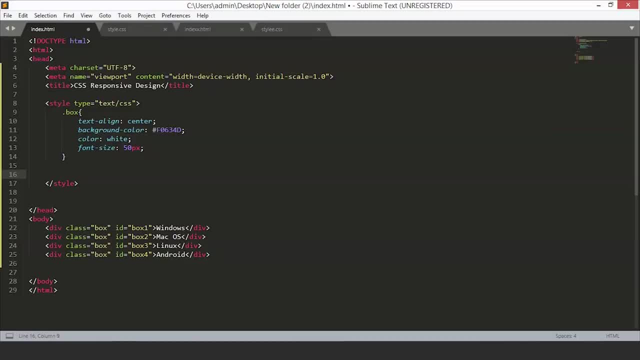 So let's start with the media queries. So media queries are used when you want to customize the website's presentation according to the user's screen size. With the help of the media queries, you can display different markers based on the device's. 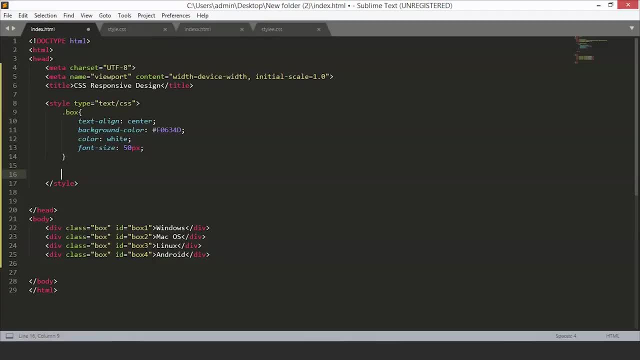 general type mobile desktop tablet, you name it. A media query is a logical operation. whenever a media query becomes true, then the related text is applied to the target element. So to start the media query, just type at the rate and media. 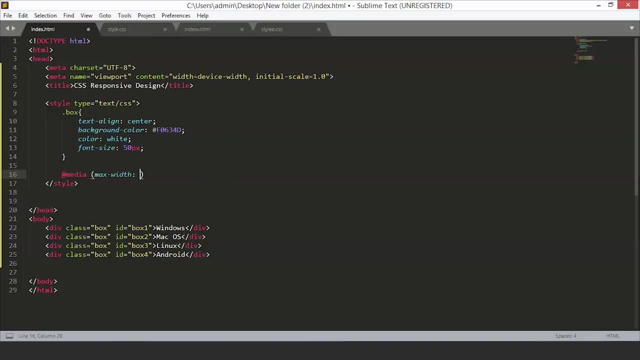 Now here we will mention the max width, to say 400px, And inside this media query we write the CSS code that should take in effect when this condition is satisfied. So here we will set the box 1 to display block. 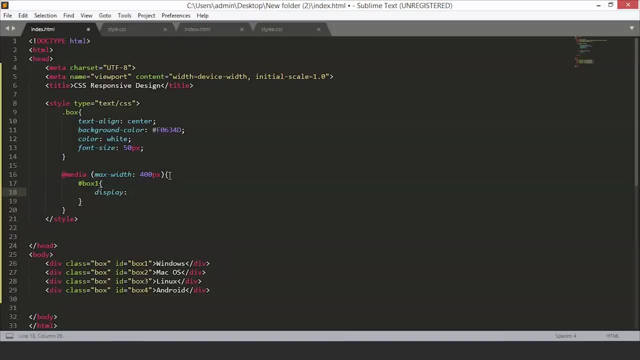 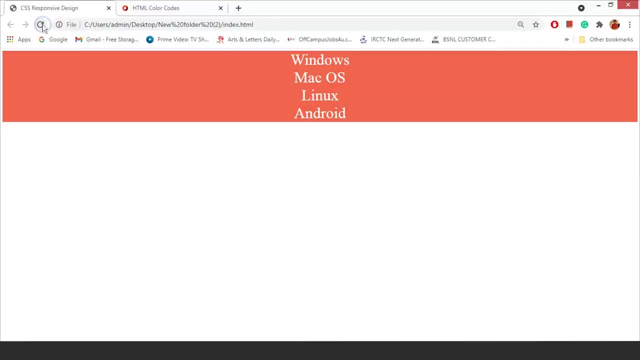 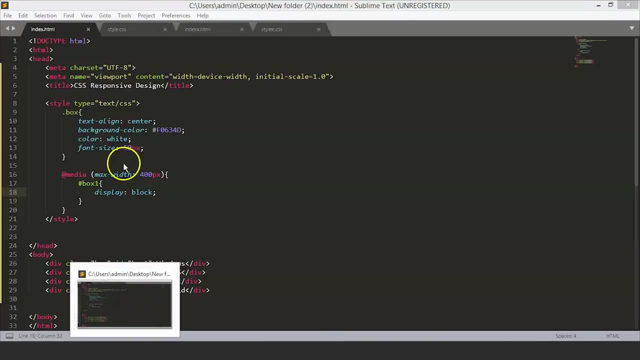 Now if you go back to the page and you refresh, you see nothing happens Because we have not made this display to none. So first go back to the CSS code and set here display to none. Now you can see we don't have any display here. 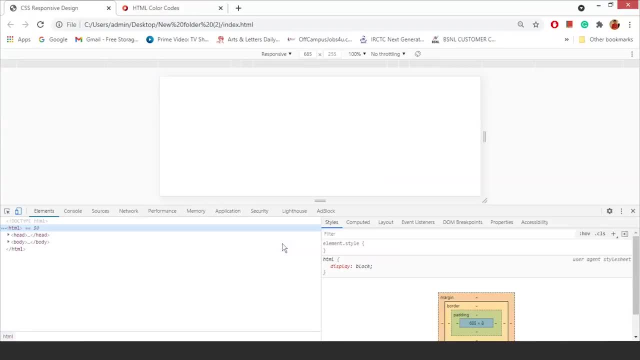 So let's inspect the page first, So you will see. we have our contents here Now you can see. this is the layout we are currently using, So we are going to set the box ID 1, width is 685px, into height 255px. 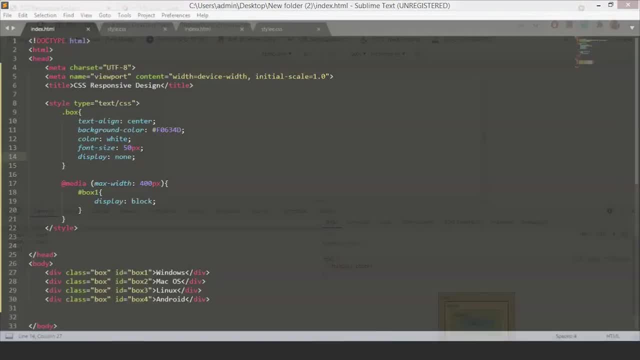 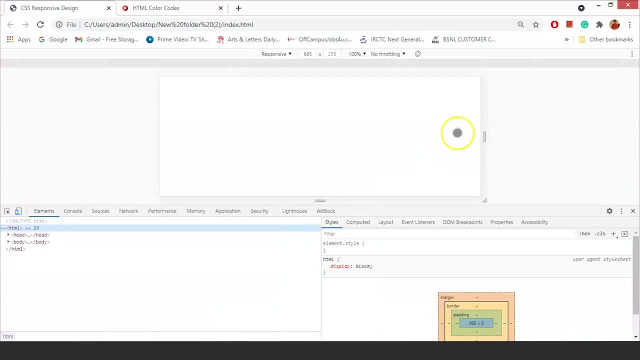 Now we are setting the max width to 400px. This means, if this width decreases to less than 400px, how this CSS code will kick in. So let's decrease the width here. So, as you decrease this width, you will see, as soon as it gets less than 400px, how CSS. 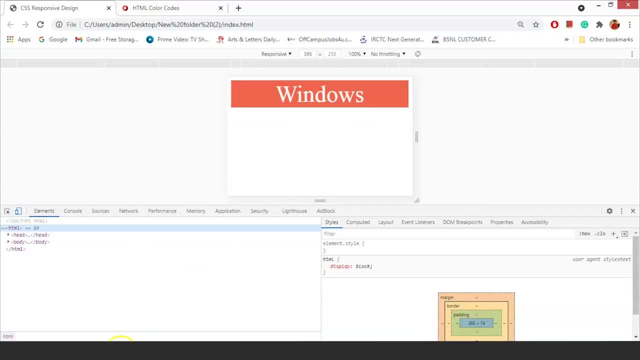 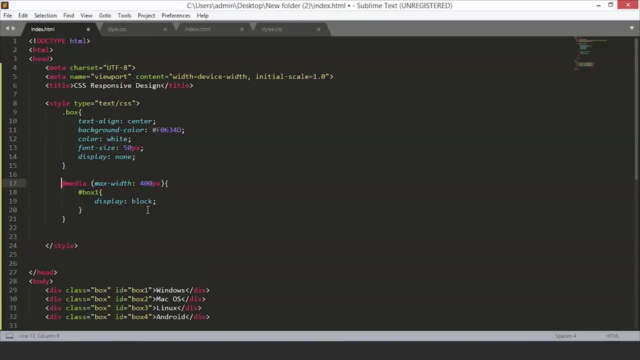 kicks in. So we have our windows displayed here, Which is the box ID 1.. So this is how the media query works. Let's add some more media queries to understand it better, So let's copy this code down: 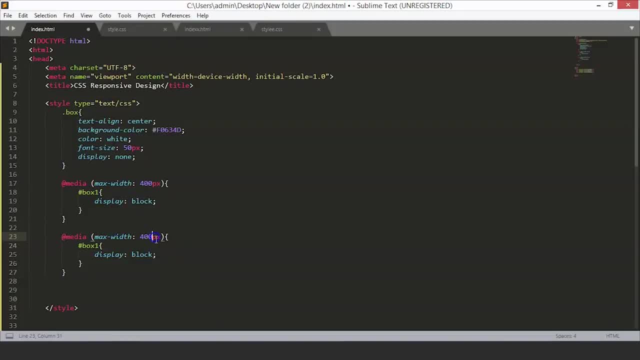 So now let's set this minimum width to 401px and maximum to, say, 600px. Now, when this condition is true, let's say we want our box 2 to display block with color green. So let's set the background color here to, let's say, green. 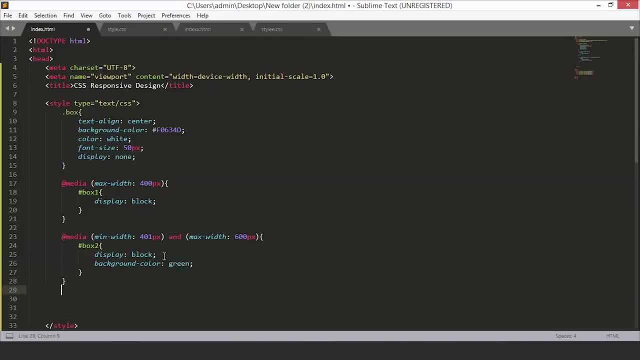 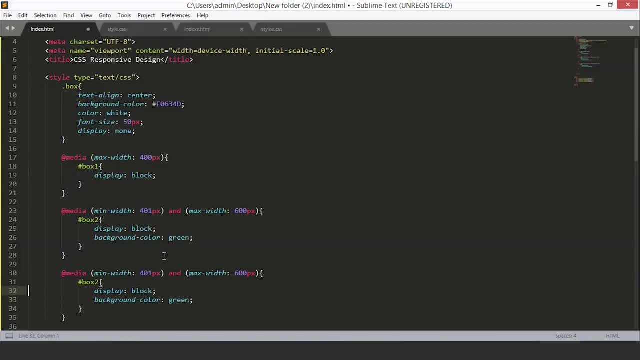 Now we have our box 2.. Now we have our box 2.. Now we have our box 2.. Paste it here. So when the width is from 601px to say 800px, So we will set the box 3 display to block and color to say pink.